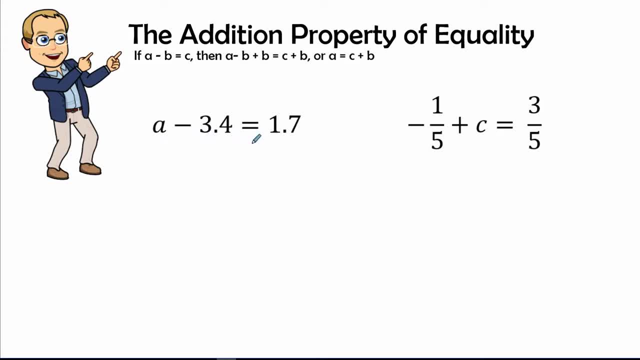 a minus three and four-tenths is equal to one and seven-tenths. Now we look at the constant that is attached to the variable. So what is attached to the letter a, Three and four-tenths, And how is it attached? It's attached with a negative sign or a subtraction sign. So we ask: 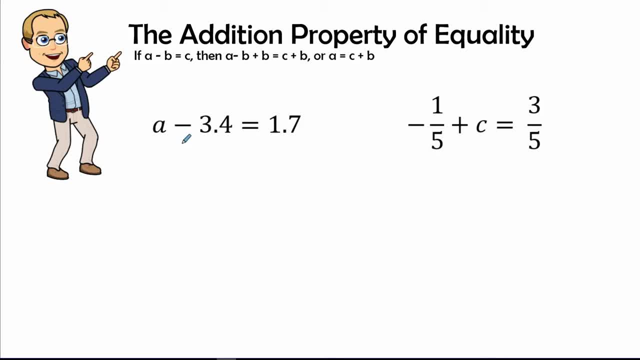 ourselves what is the opposite of subtraction, And that would be addition. So we are going to add three and four-tenths, And so we are going to add three and four-tenths. And so we are going to add three and four-tenths to both sides of the equation. So when we go ahead and add three and 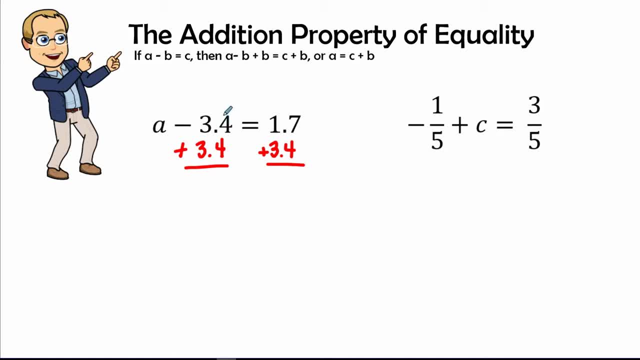 four-tenths to a negative. three and four-tenths. they're inverses of each other and they equal zero. So we're going to bring the letter a, or our variable a, down, set it equal to, and then we are going to add one and seven-tenths and three and four-tenths. Seven plus four is eleven. 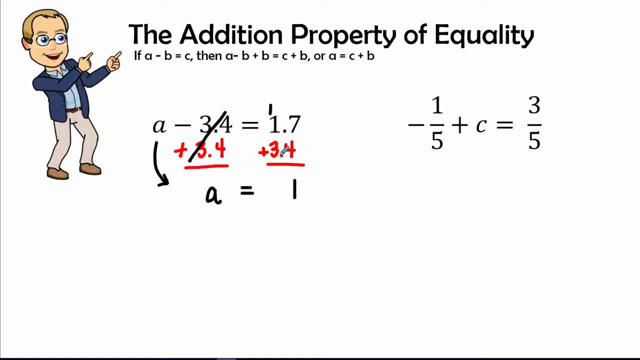 We are going to carry our one Three and one is four plus the one is five. Now it's not a equals fifty-one. We have to make sure we keep our decimals in line as best as we can, and we need to insert it into our answer. So really, instead of a equals fifty-one, the correct answer is a equals. 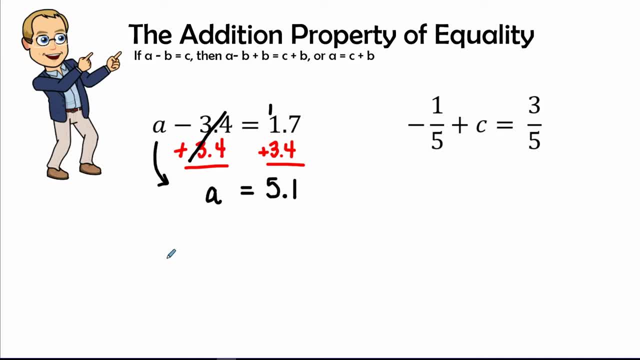 five, point one: Let's go and check our work. So wherever I see a variable, a, I'm going to write a, I'm going to put 5.1.. So 5.1 subtract or minus 3.4 is supposed to equal 1.7, or one and seven. 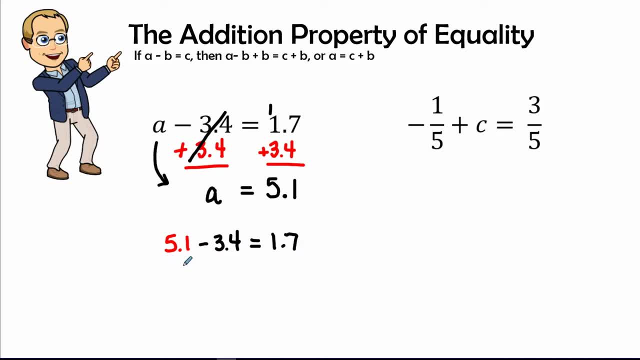 tenths. So when we subtract we see that five and one tenths minus three and four tenths is one and seven tenths. And sure enough, they check and we double checked and we guarantee that we have a correct answer. Now in the next problem, we have negative one fifth plus C. 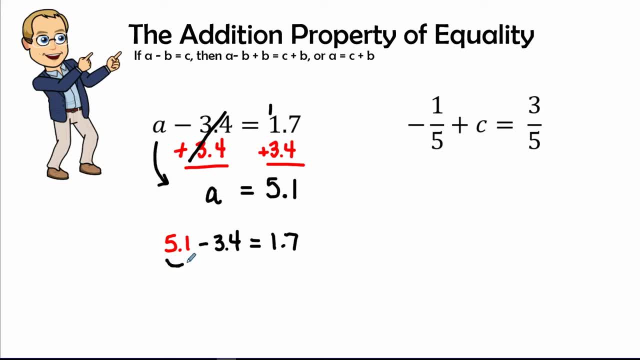 So when we subtract we see that five and one-tenths minus three and four-tenths is one and seven-tenths. And sure enough, they check and we are double-checked and we guarantee that we have the correct answer. Now in the next problem, 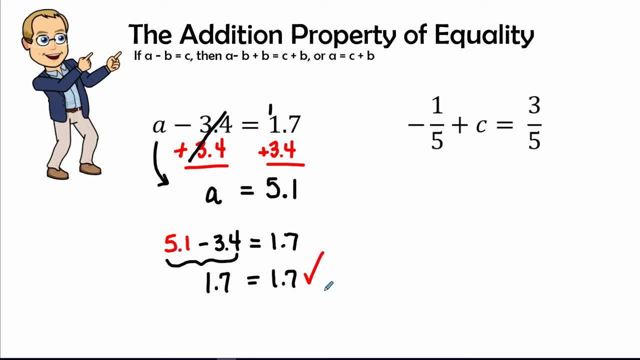 we have negative one-fifth plus c equals three-fifths. So we ask what is attached to the letter c or the variable c? It is attached by a negative one-fifth, So the inverse of a negative one-fifth is a positive one-fifth. 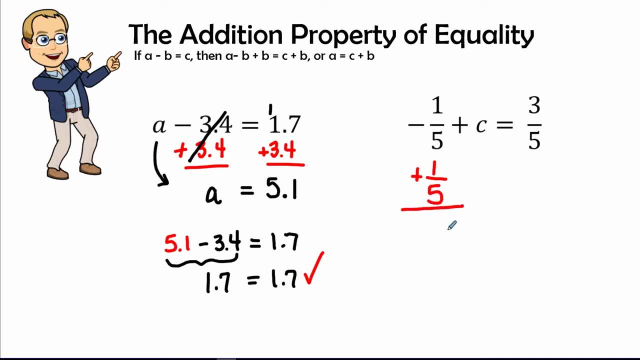 So we are going to add both of those together And negative one-fifth and a positive of one fifth is an inverses, so it equals zero. So now we have c by ourselves and I went ahead and I forgot to add this one fifth to the other side. Remember, in the addition property. 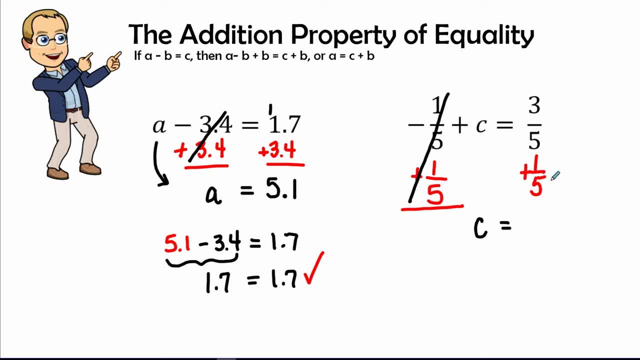 of equality is what I do on one side of the equation. I'm going to do on the other side of the equation. So I see, right here I have two fractions with the same denominators, or like denominators. therefore, I can just go ahead and add the numerators. Three plus one is four. 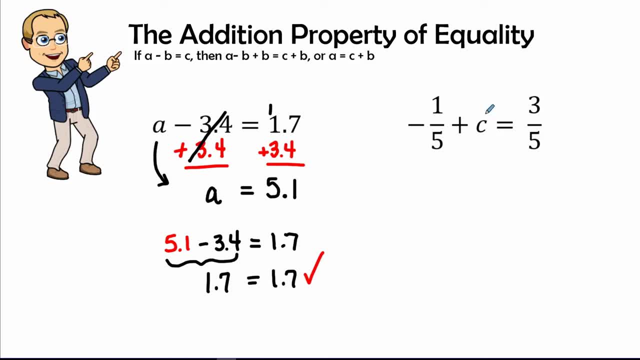 equals three fifths. So we ask what is attached to the letter C or the variable C? It is attached by a negative one fifth. So the inverse of a negative one fifth is a positive one fifth. So we are going to add both of those together: A negative one fifth and a positive one fifth. 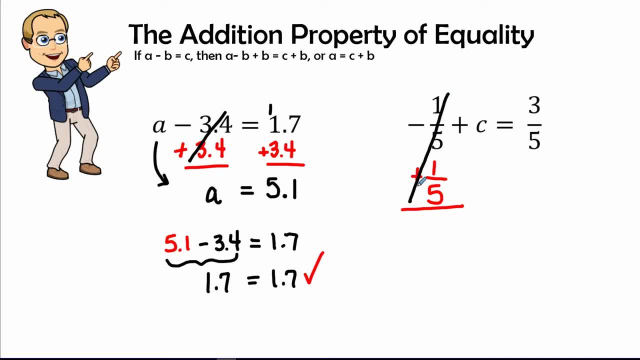 is an inverse, So it equals zero. So now we have C by ourselves And I went ahead and I forgot to add this one fifth to the other side. Remember, in the addition, property of equality is what I do on one side of the equation. I'm going to do on the other side of the equation. 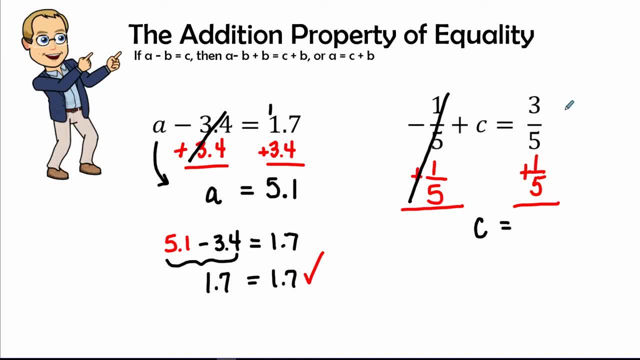 So I see, right here I have two fractions with the same denominators, or like denominates. Therefore, I can just go ahead and add the numerators. three plus one is four And I keep my denominator of five. All right, let's go ahead and check our work. So here we go. I have a negative one, fifth. 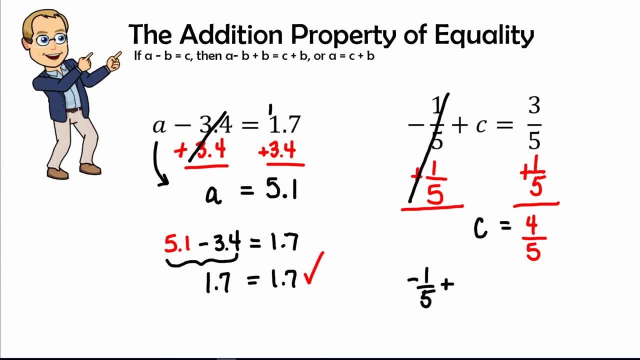 plus C. We know that C is supposed to, So wherever I see a C, I'm going to insert a. four fifths, Therefore, and it's all supposed to equal three fifths. So when I combined my numbers together, I haven't. I know that I have like denominators, So I'm going to have a like denominator in my 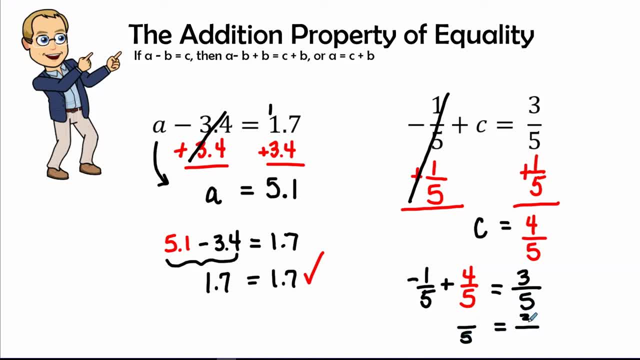 answer. And this is supposed to equal three fifths. So let's check it out. I have a positive four and a negative one, So four, and I'm going to add a negative one that gives me three. So, sure enough, three fifths equals three fifths. Therefore, C equals four fifths. is the correct answer. 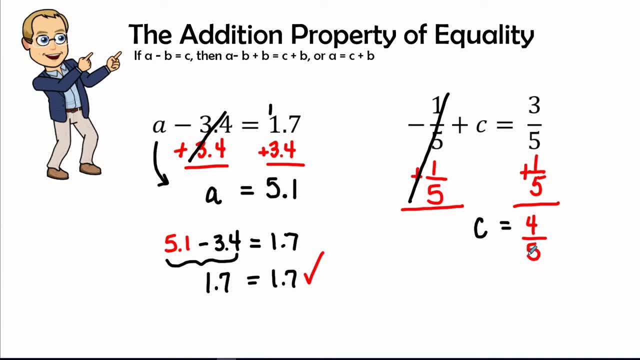 and I keep my denominator of five. All right, let's go ahead and check our work. So here we go. I have a negative one. fifth plus: we know that c is supposed to, so wherever I see a c, I'm going to insert a. four fifths: 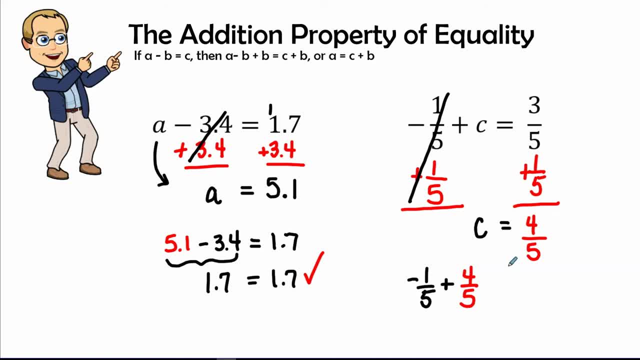 and therefore, and it's all supposed to equal three fifths. So when I combined my numbers together, I have it. I know that I have like denominator, so I'm going to have a like denominator in my answer, and this is supposed to equal three fifths, so let's. 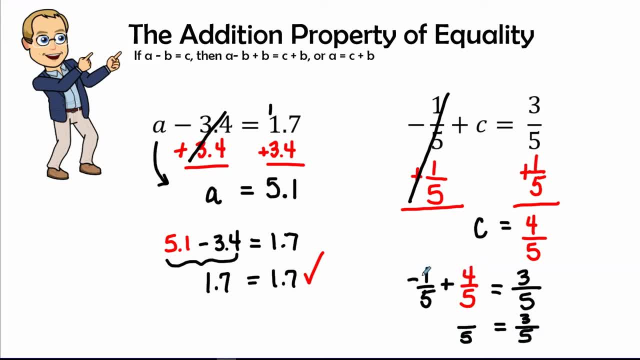 check it out. I have a positive four and a negative one, so four, and I'm gonna add a negative one that gives me three. So, sure enough, three-fifths equals three-fifths. therefore, c equals four-fifths is the correct answer. Subtitles by the Amaraorg community.